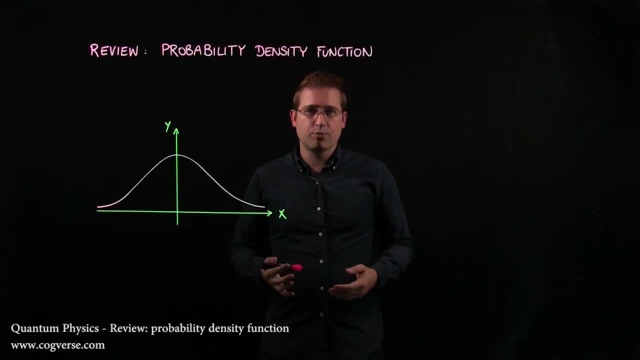 Before we move on to the Schrödinger equation, let's briefly review probability density functions. A function, f, is said to be a probability density function if it is continuous and positive on its domain, can be integrated over its domain and, in addition, is such that the probability 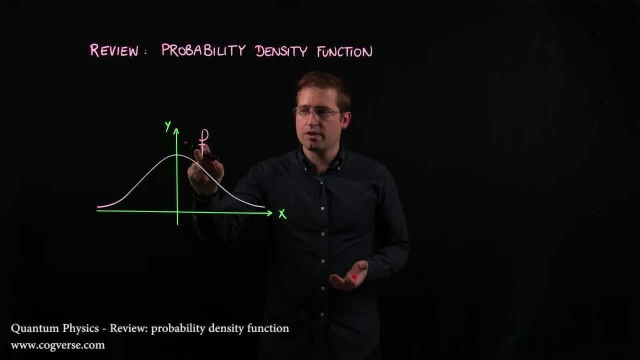 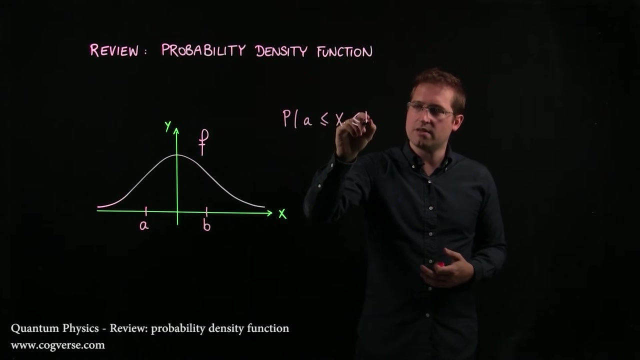 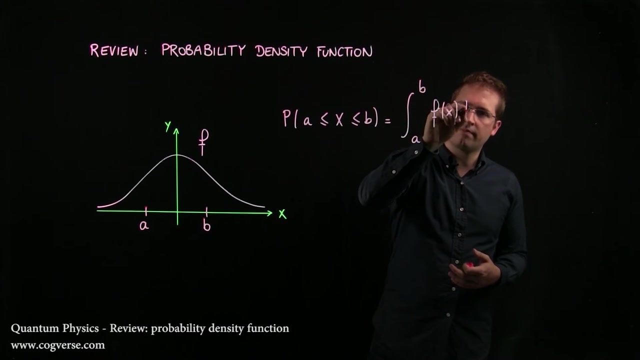 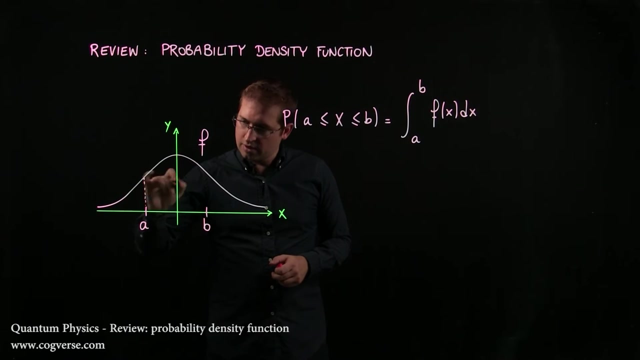 that the random variable big X, associated with the probability density function f, take on a value between a and b, two real numbers, is equal to the integral from a to b, of f, of x, dx, And that integral, if you remember, is exactly equal to the area of this region. 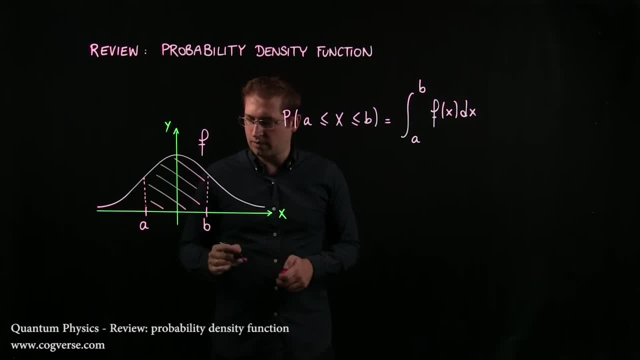 here. In addition, because this is a probability, we know that it's probably greater than zero, but less than one, And we know for sure that the random variable big X will take on a value that is between minus infinity and plus infinity. So f will also satisfy the condition that the integral from minus infinity to plus infinity of f of x, dx will be equal to the integral from minus infinity to plus infinity of f of x is equal to one because for sure x will take on a value between minus infinity and plus infinity. 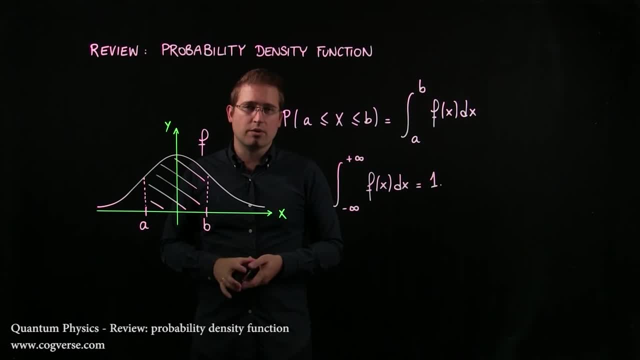 Now, why is this important? Well, it's important because once we do the Schrödinger equation, we'll find that the solutions that are called wave functions are in fact the best possible description of the quantum state of a particle, And usually the solutions are denoted by: 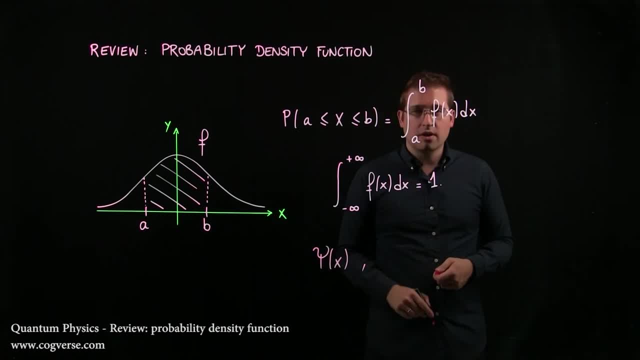 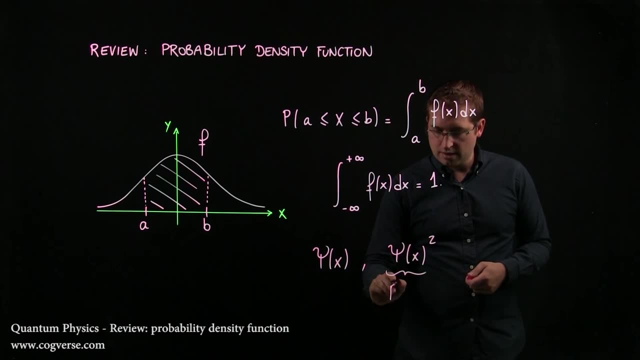 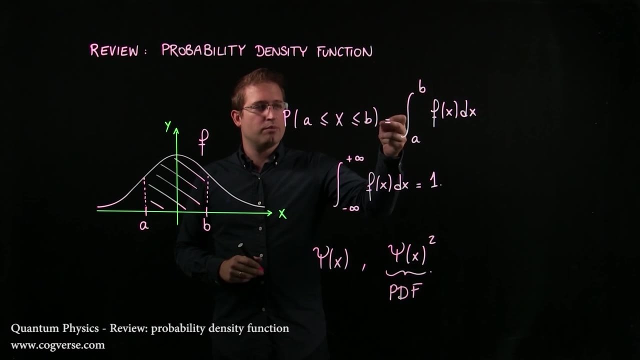 psi of x. But if we take psi squared, Then psi squared is a probability density function And therefore it's going to be important to remember both this property and this property when it comes to psi squared.